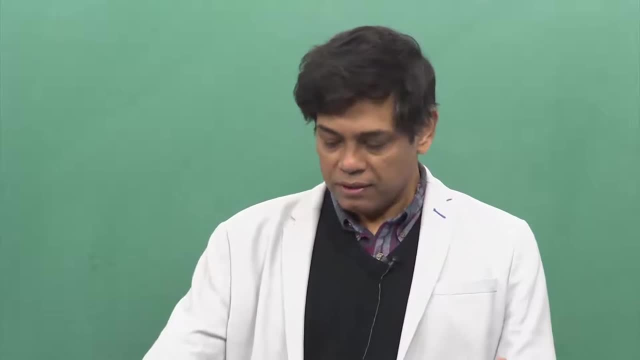 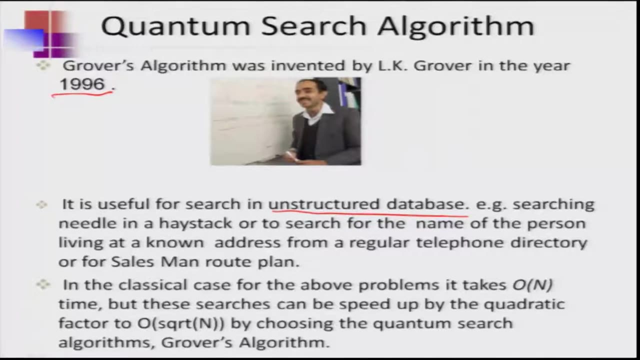 faster by using classical structures. However, for example, to search a needle in a haystack or to search the name of a person living in a known address in a regular telephone directory, these are very hard problems and this can be done by using this technique. 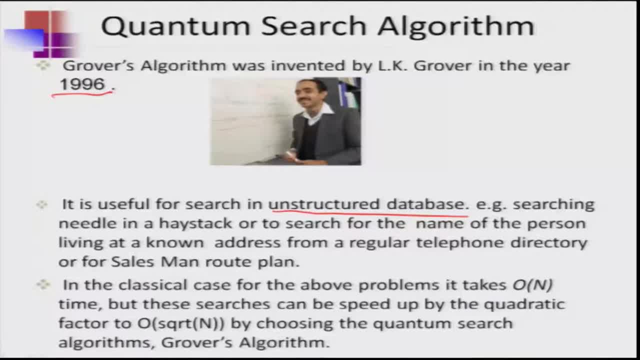 It is also applicable for salesman to find out a route, his plan for selling items. All these kinds of applications. this particular problem is applicable In the classical case. for any of these above problems it takes an order n time, but these searches can be spread up by the quadratic factor. to order square root of n by choosing: 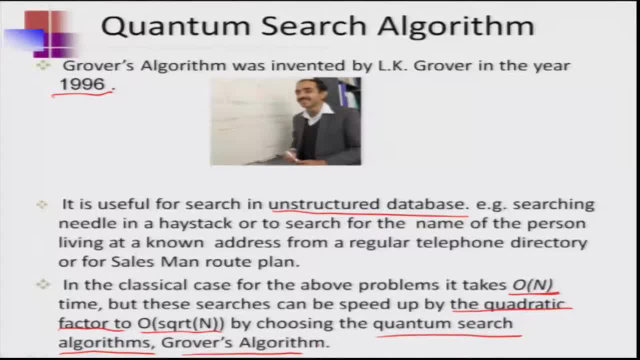 the quantum search algorithms, which is also known as the Grover's algorithm. The basic idea behind this algorithm is to come up with a technique which is not going to look at the data set one by one, but it is going to do it in a quantum way, so that 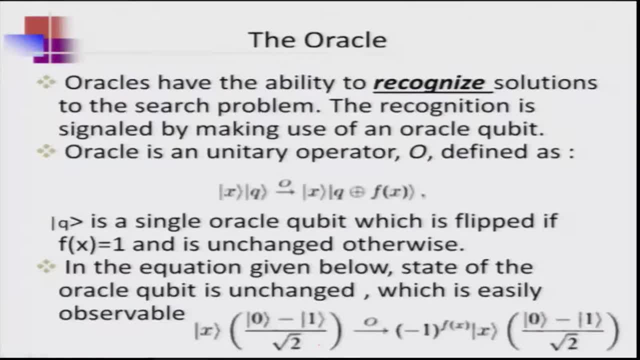 it is done at a much faster rate. that is the basic idea. The oracles have the ability to recognize solutions in the search problem. The recognition is signaled by making the use of an oracle qubit In this particular case, because it is going to be quantum case. 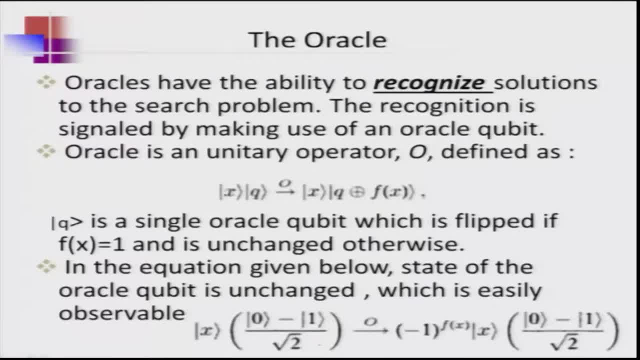 So the oracle will be an unitary operation which can be defined as the operation of the qubit on, so defined as the operator O which works on the set that we are looking at, such that we create a functional dependence of the two, Where Q is a single oracle qubit which is flipped if the function is equal to one and it is. 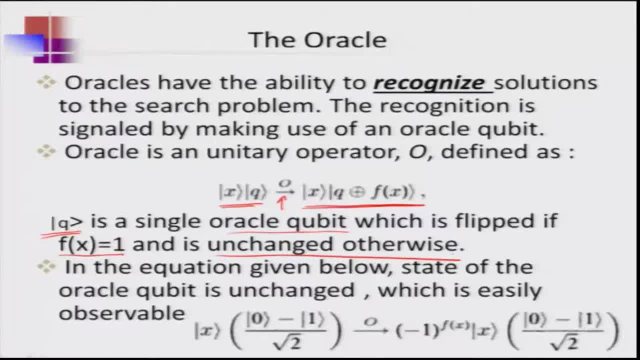 unchanged otherwise. So, basically, the setup of the oracle as an unitary operator can be defined in this particular way where, by using the single qubit Q, which is our oracle qubit, the idea is to make it flip When the function changes. that is when I have found the solution, the search that you are. 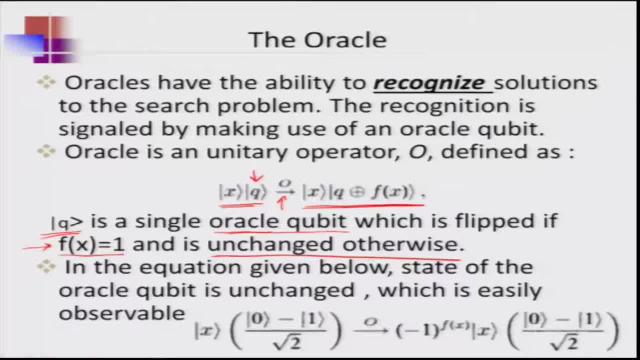 looking for or it remains unchanged. So as long as the operator does not give the result of being flipped, we continue doing the process. We look for the searching In the equation given below. the state of the oracle qubit is unchanged, which is easily observable. 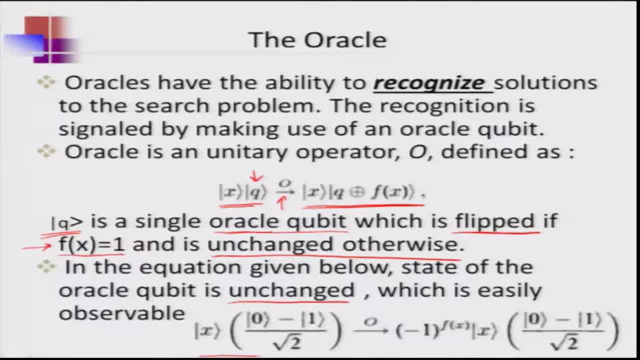 So, for example, Q is a single oracle qubit. For example, when you take a state like this and we finally see what is going on with it, the oracle qubit keeps remaining the same, which means that I can keep on using it over and over again. 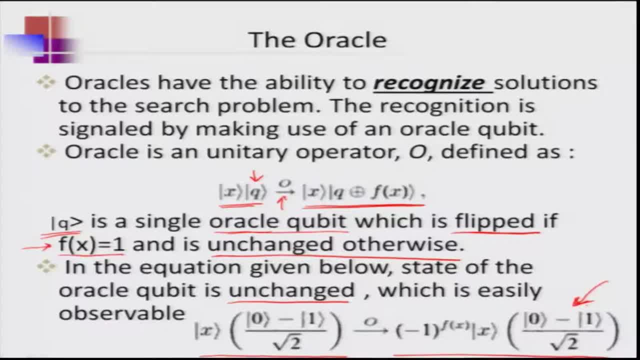 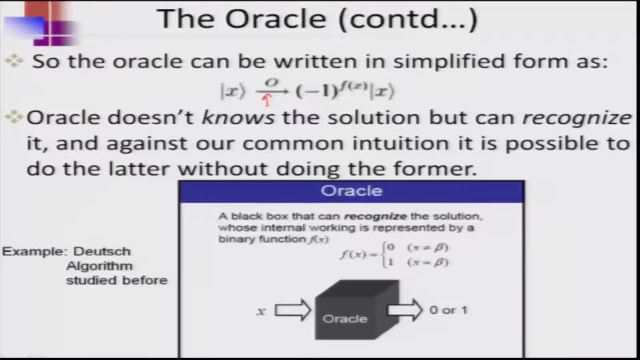 So that is the idea behind an oracle: that the oracle should keep on reporting the right solution in spite of not changing. Okay, In a simplified form, The oracle can be written in this form, where if you have the qubit, then you are going to. 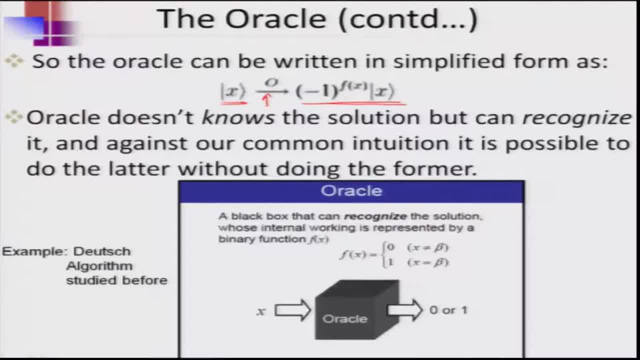 have the function which is going to have this minus 1 f of x to the power of f of x times the qubit that we are looking for. So, in other words, the oracle does not know the solution but can recognize it and, against our common intuition, it is possible to do the later without changing the former. 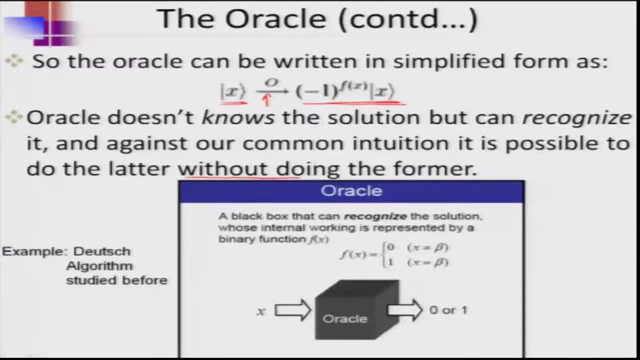 So the most important part here to remember is that it does not change the oracle qubit. An example of that you already have- we have seen it before in case of the doish algorithm, where the black box, which we call the oracle, is the one which can recognize the solution. 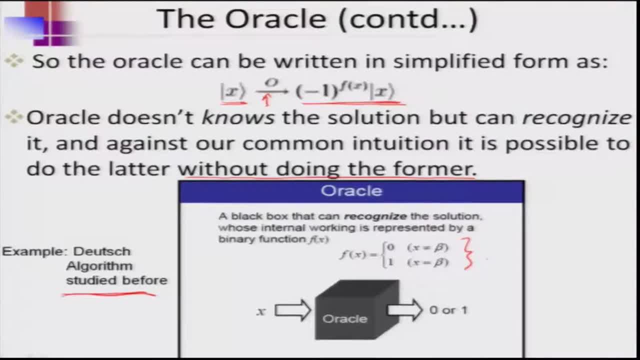 whose internal working is represented by a binary function. So once we put it through the oracle, The Functional form, It will be giving out either 0 or 1, although the oracle keeps it the same way. So basically, I can keep using the oracle over and over again and get the algorithm go. 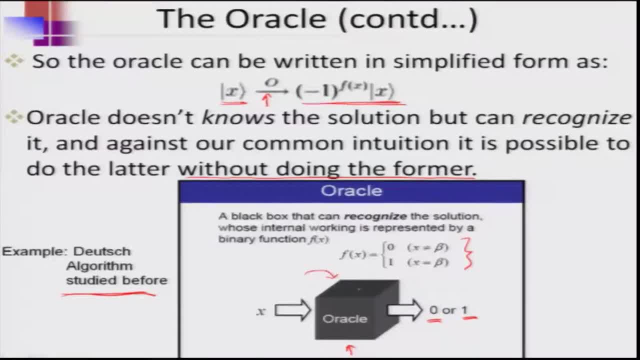 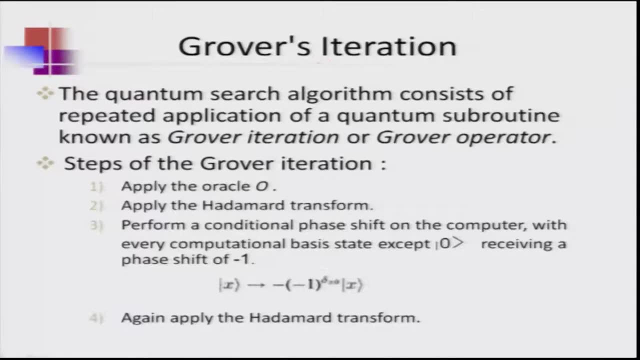 And this is one of the ideas of making sure that I can- we can go ahead and apply quantum concepts to develop a faster way of doing the computing. So now, given this background, it is understood that there will be Multiple iterations that will be necessary to get the solution from this search algorithm. 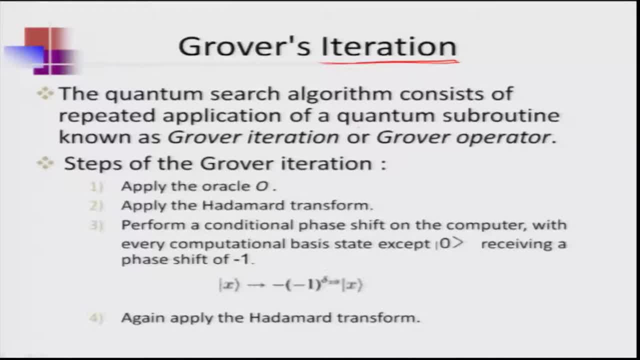 So the quantum search algorithm consists of repeated application of a quantum subroutine known as Grover's iteration or Grover operator. In the classical sense, when we were supposed to search, we were supposed to go through each and every data point to be able to get to the solution. 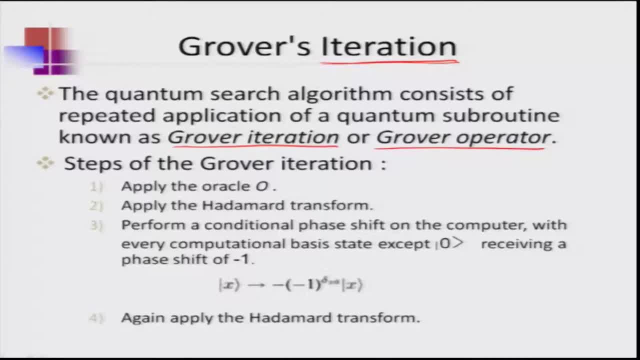 In this particular case, It consists of repeated application of the quantum subroutine Instead of having to look through each and every data. That is the basic idea. So, in other words, the steps of the Grover iteration is: number one is to apply the oracle O So 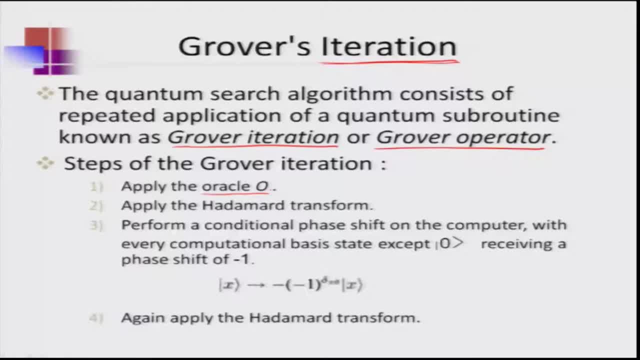 first of all, we have to set up an oracle, as we discussed, in such a way that it can recognize what we are looking for, the search. Then we need to apply the oracle, Apply the Hadamard transform. Now, Hadamard transform is something which we have. 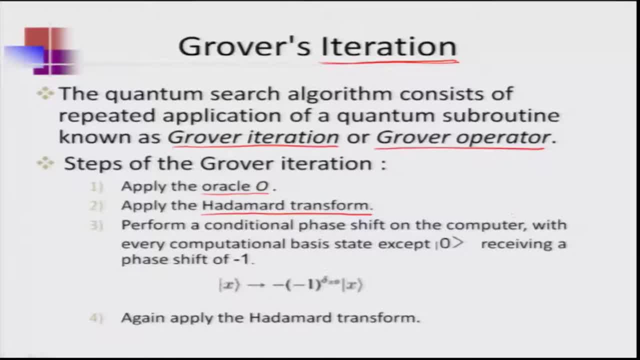 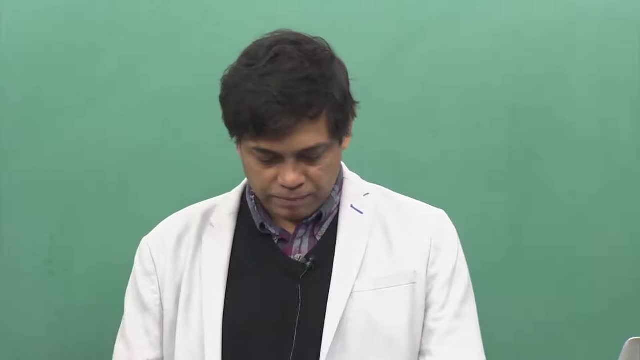 Applied before, which we have learnt about before. This transformation essentially takes the qubits and mixes them up. So if you take two qubits situation, then it will give equal weightage and put them together. That is the idea of Hadamard transform. 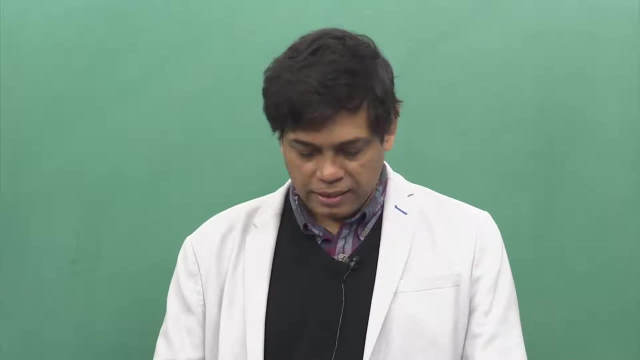 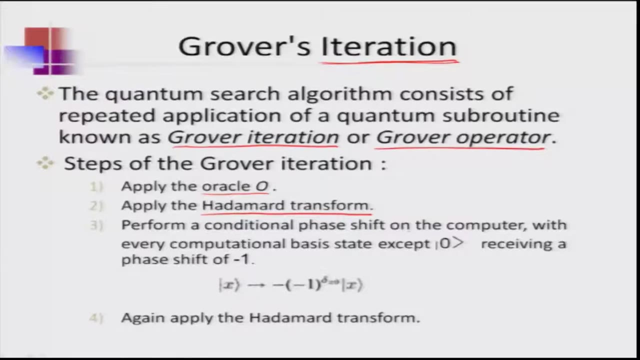 So we will again revisit that to iterate our memory. But generally this is how the transform is. Then we will do a conditional phase shift on the computer with every computational bit set except the zero receiving a phase shift of minus one. So that is how we will take our data set from X to X with this particular functional dependence. 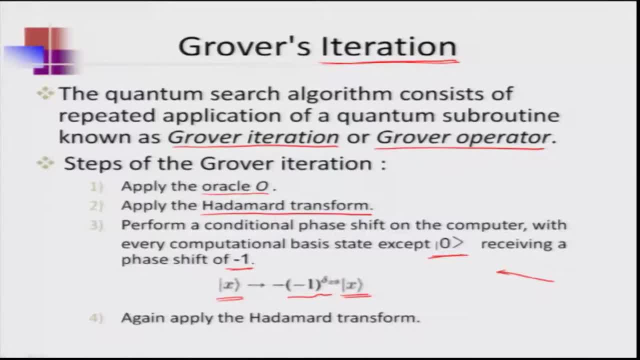 where we will get this. So this is essentially inversion about mean. So in essence, this conditional phase shift on the computer, which every computational basis set except zero receives a phase shift of. this is almost like inversion about the mean of the entire data set. That is what we will do, and then again we will apply the Hadamard transform so that 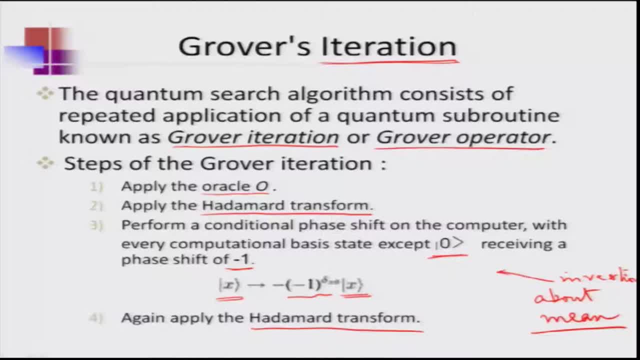 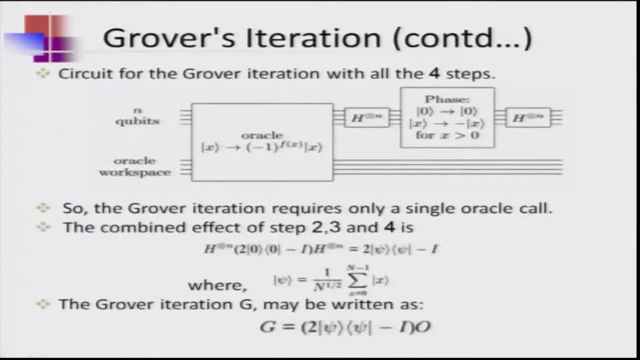 we can get back to the data set as we had before and be able to understand what we have just done. So these are the steps. So, in other words, if you want to write it in terms of the circuit, the circuit for the Grover iteration with all the four steps that we just mentioned looks like this: 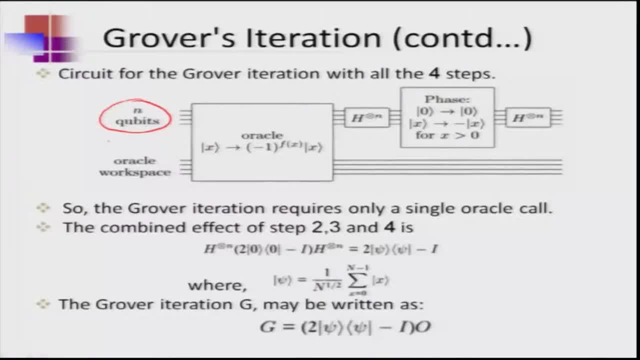 We have the n qubits which need to be loaded up. Then we have the oracle workspace that we have just discussed. Once we put this together inside the oracle, it is essentially undergoing a transform, where the functional decision as to whether the function value is one or not is being found. 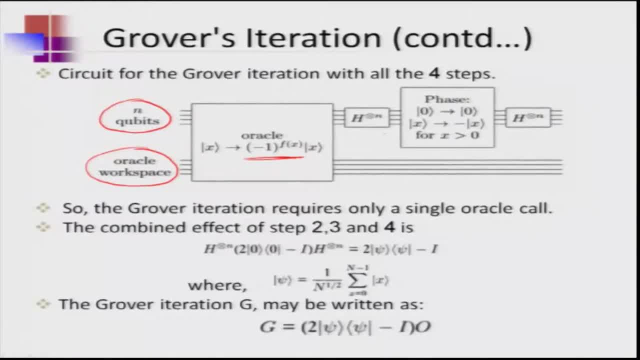 so that you apply the oracle and get the solution And then you again do a Hadamard transform. You do the Hadamard transform, apply the phase shift around the mean About zero- It is the same. It means that it is actually doing an inversion about the mean- and then apply the Hadamard. 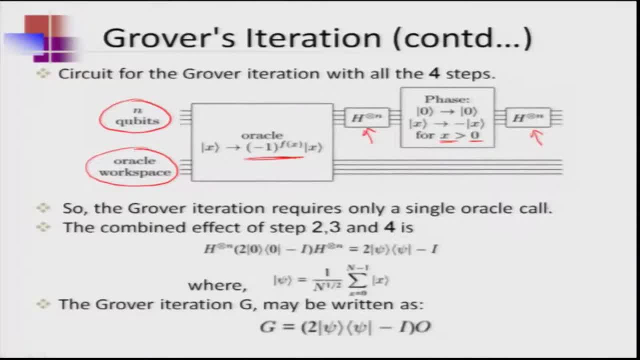 transform again. In some sense, therefore, the Grover's iteration requires only a single oracle call, Because once you have set it up, put it in the oracle workspace. You just need to set it up once to be able to find out whether you have got the solution. 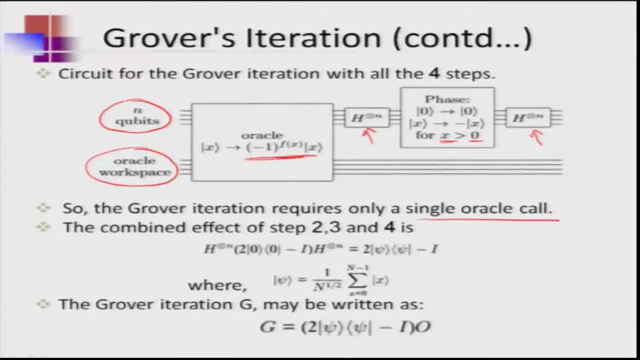 or not. The combined effect of steps two, three and four- So two, three and four, So this was our first step- Is that we have applied a Hadamard on this initial set and a reverse Hadamard And, depending on if you are doing it once or that many times, we will have it to the 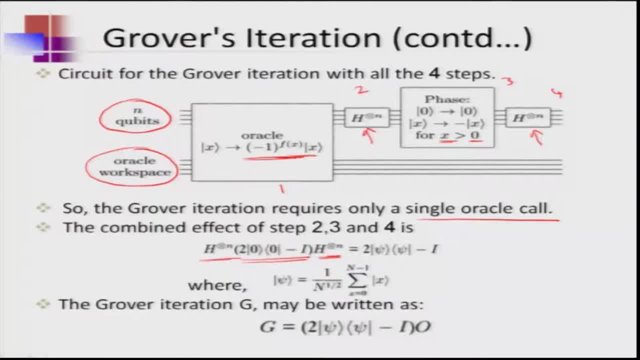 same degree. This operation applied that many times so that we are able to get the solution And a wave function, therefore, is represented by this one over- this is a normalized case- one over N to the power half x vector. So the Grover iteration G then, therefore, can therefore be written as this particular set. 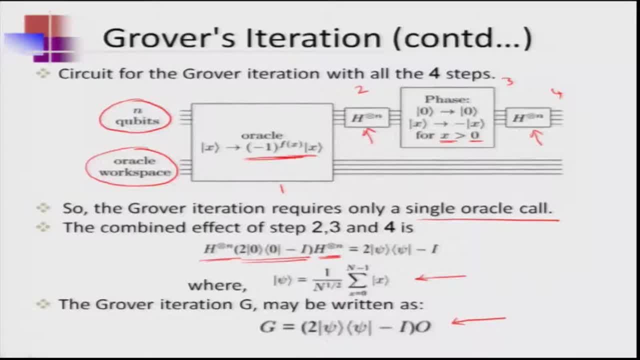 G is equal to two times x. Okay, Two times wave function, put in the different ways, minus i, and then the operation that we are applying, which is the oracle operation. So this is the iteration process that we will continue, and once we keep on doing this iteration, 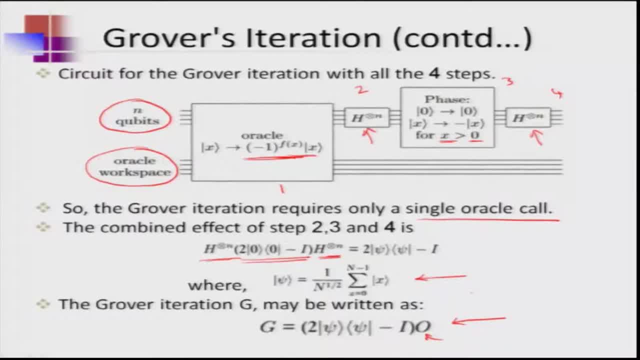 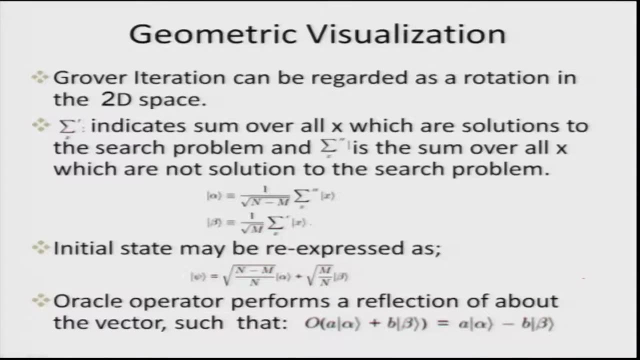 we will be finally getting the solution. So this is the iterative way of doing this particular approach of Grover's algorithm. Okay, Thank you, Let us see how it looks. We can also visualize this geometrically, because many a times this entire process can be understood. 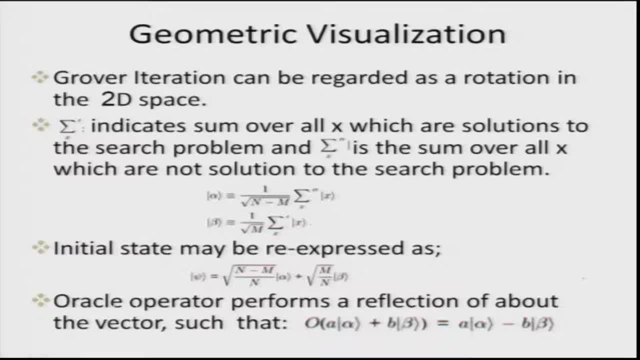 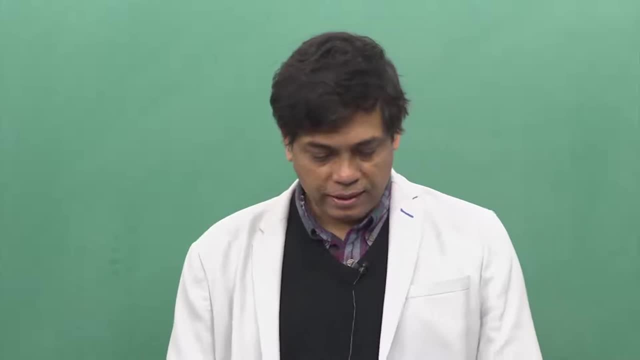 much better if we visualize this geometrically. So this can in that sense be regarded as a rotation in the 2D space, And that is a perhaps a much more intuitive way of understanding how this is going In this process We can. 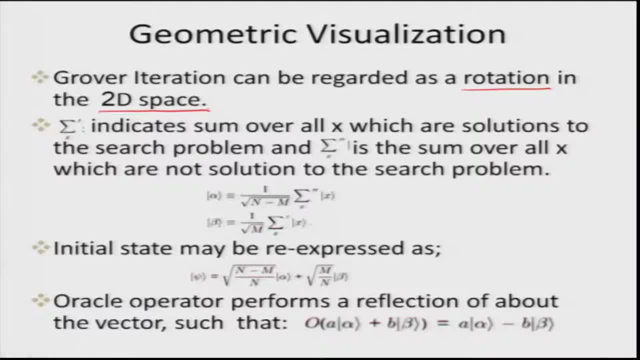 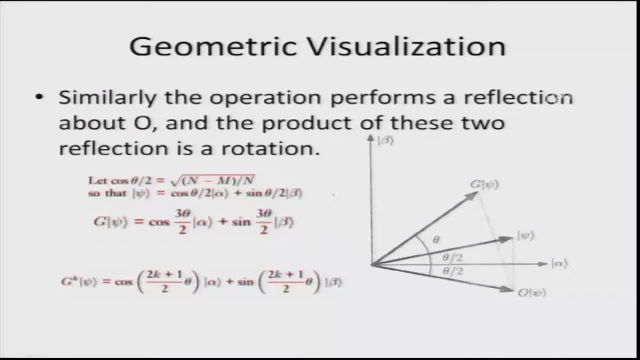 We can actually look at this entire process again in the same way. Maybe I should show the figure before I go ahead with this. So here is the geometric visualization where we have this 2D axis, and this is my. this is the state that we are looking at. 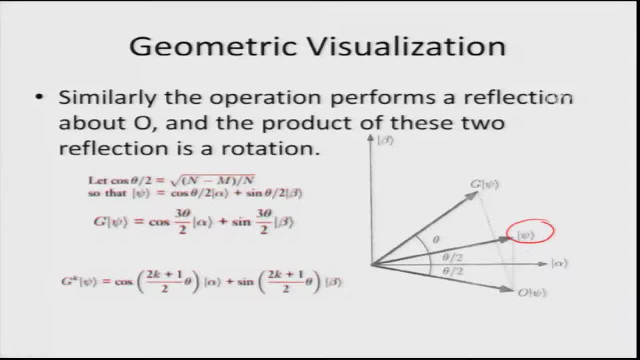 So this is my wave function and, depending on whether I am rotating it, Which, Which, Whichever way, So So this is my state alpha, This is my state beta. These are the two components of the wave function that I have. 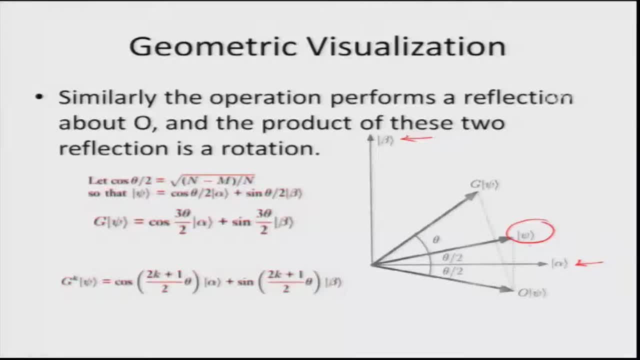 Now my operation can essentially take it down one way or the other and around one of the mean positions. So if alpha is my mean position, I can have this go- Okay, Down by theta by 2 or theta by 2 in either direction, or we can go up the entire direction. 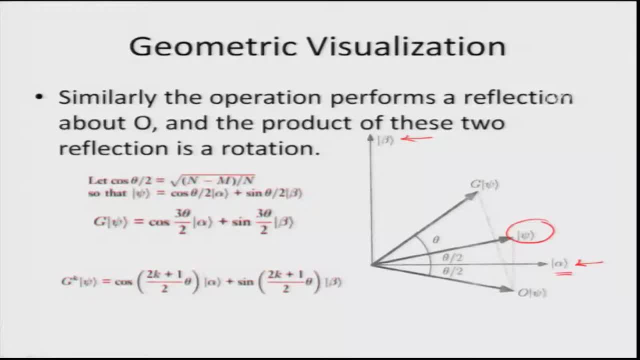 by theta. So basically it is a reflection about the wave function that we can go in either direction. The operation performs a reflection about O and the product of these two reflections is a rotation. So this is my operation, which is essentially doing the reflection and as a and the product. 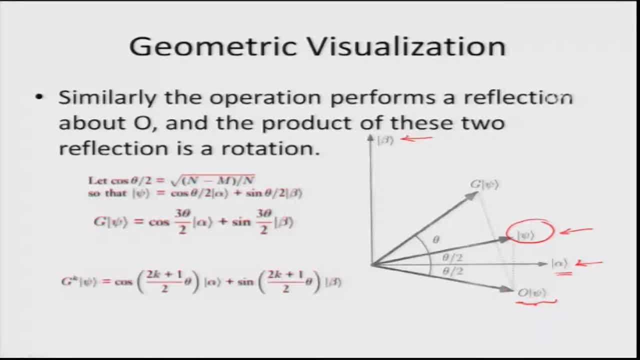 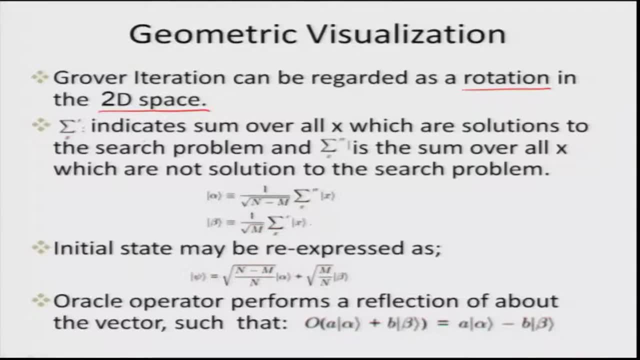 of these two reflections is a rotation. Let me again go back to the earlier slide to essentially indicate all the mathematics associated with this: The sum over all the x which are the solutions to the search problem, and double prime, say summation prime of x and summation double prime of x are the two sums. 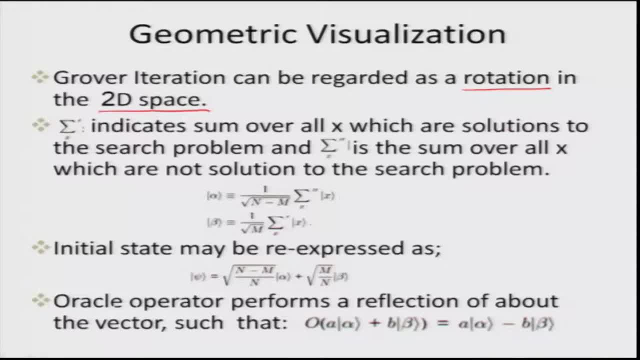 One of them is the one which is solutions of the search problem and the other one, double prime one is the sum over all x- which are not solutions to the search problem. So there are two cases, Basically: one which is the case with the solution and the case which is without the solution. 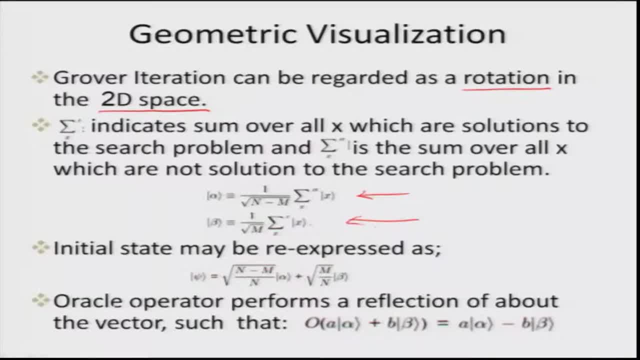 Then we can set up two different states, say alpha and beta. This is what I was trying to represent when I went back to the other picture, So we will go back to this after setting it up. now See, alpha and beta are the two cases where we have set up between solution versus no. 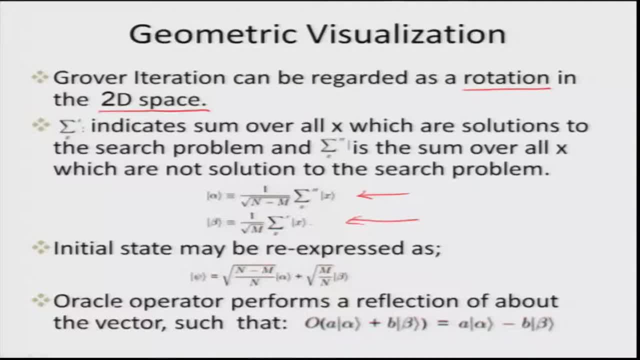 solution. So the initial state may be represented As something which is a superposition of these two conditions, where we have the solution and we do not have the solution. And that is the way how you can read it. And then the oracle operator performs a reflection about the vector such that it will rotate. 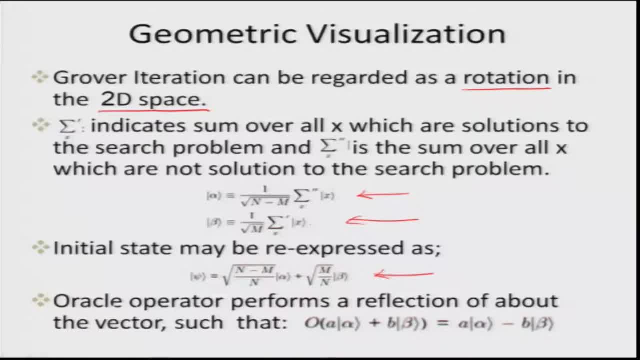 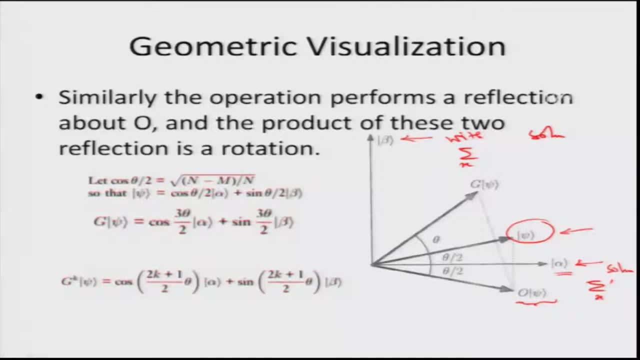 it such that we will be able to find the description of the state amongst that. between the solution case, This is the one which does not have the solution case and based on these we can get to our solution. So we have a solution case, with solution is this one, and without solution is the one where. 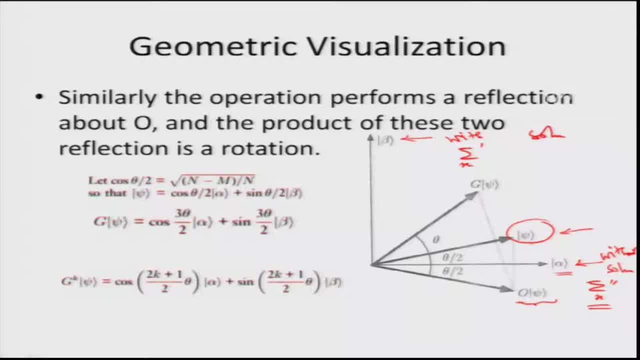 the alpha. So now my wave function is somewhere in between alpha and beta, which basically means that it is a superposition of the two or having contribution from both of them. See, if we consider an angle, An angle theta, such that the cosine theta by 2 is the weightage factor n minus m over. 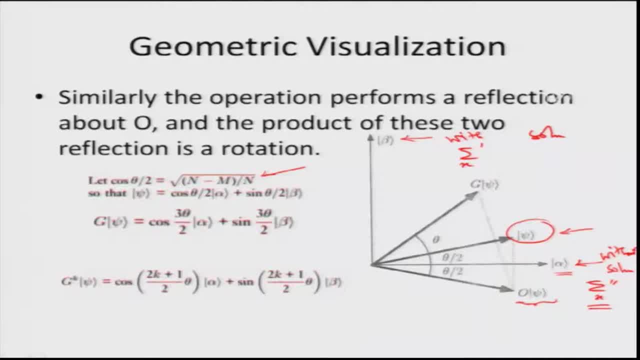 n root over square root, Then we can tell that the wave function is cosine theta by 2 alpha, plus sine theta by 2 beta. So that is how we have set up the, The wave function. Now the Grover application and the state essentially takes it to cosine 3 theta by 2 sine 3 theta. 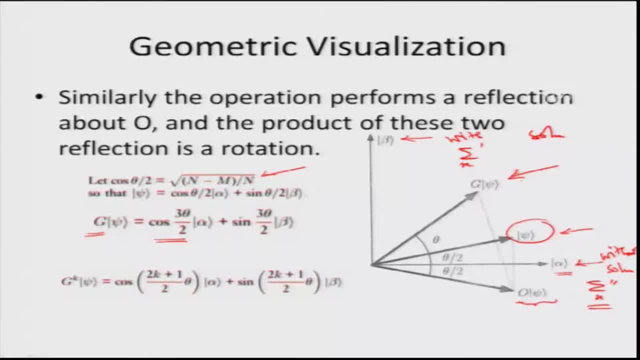 by 2, which is where this is. this is the rotation we are getting, And if we apply it k times, then this is essentially be a rotation which will bring it back and forth around that point all the time. So that is the idea behind applying the Grover's algorithm over and over again. 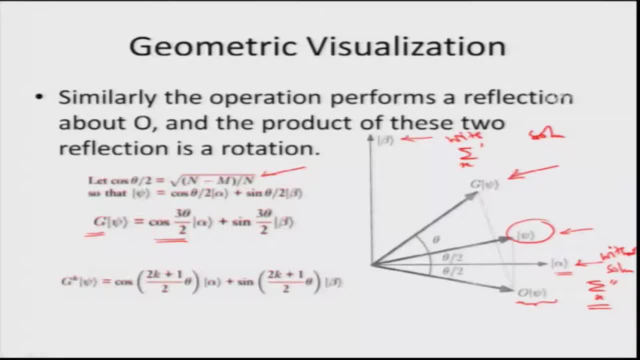 Thank you. In fact, this also tells you one very interesting thing: that there is a point- and this will do it later in a more detailed fashion- where we will show that there is a point beyond which the solution finding essentially oscillates around the actual signal. 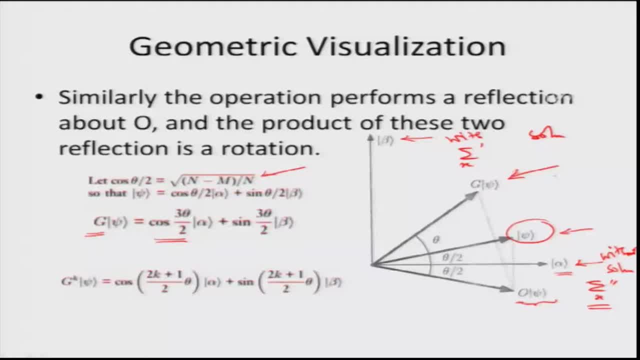 So you find out the solution by using Grover's algorithm, And if you keep on running the iteration there is nothing like further improvement or something. So the Grover's algorithm essentially oscillates back and forth around the actual solution. So once you have gotten your solution, you cannot really just say that you know you can. 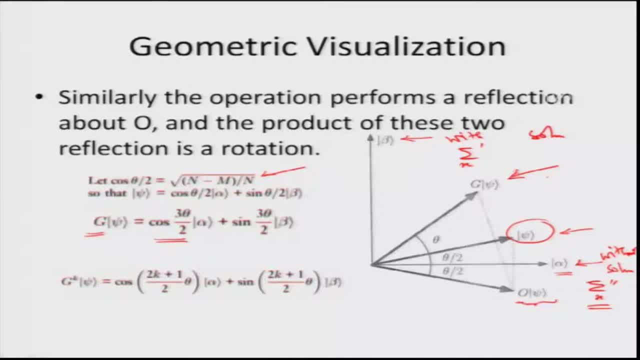 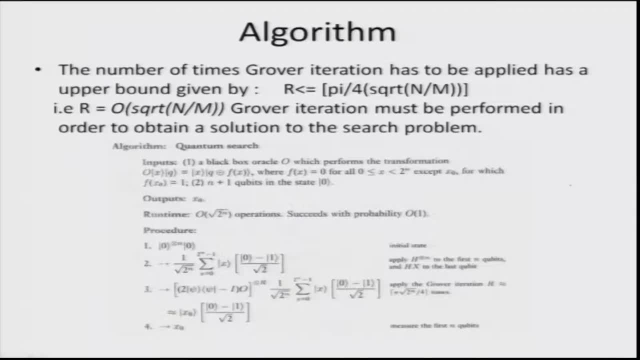 continue on doing it to get to anything better, it will just be oscillating around the actual solution. that is the idea. So, anyway, the number of times the Grover's iteration has to be applied has an upper bound, therefore, Beyond which it essentially means that it is just the back bound. 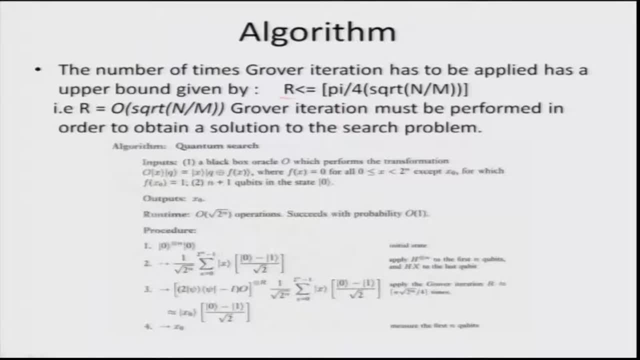 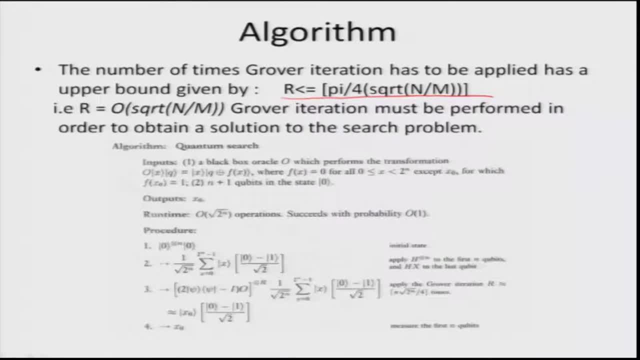 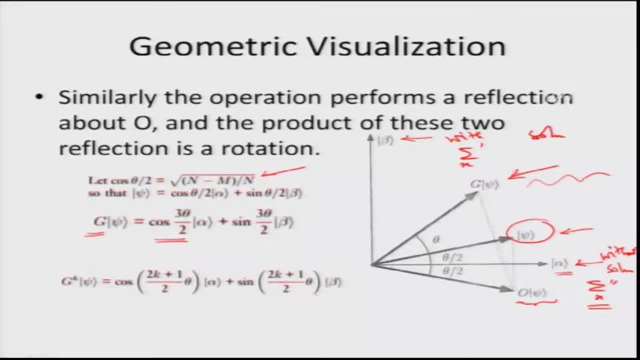 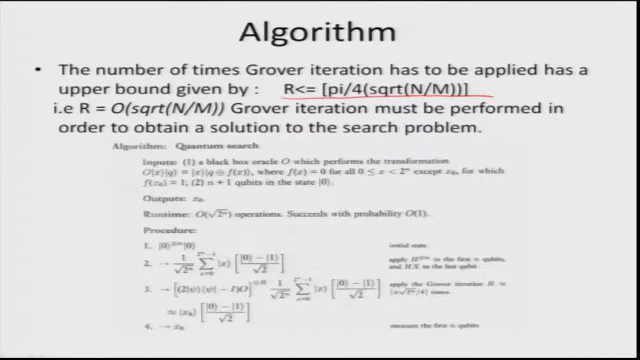 from the equations that I just wrote in the last slide. So if you apply this, how many times do you apply and do you get a number beyond which it has no meaning? So that is the value that you can actually come down to: pi over 4, square root of n over. 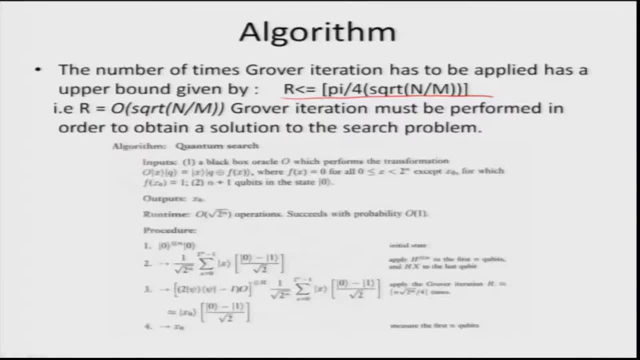 m. That means that my r has the order of square root of n over n. Grover's iteration must be performed in order to obtain a solution to the search problem, and that takes an order which is square root of n over m. So the basic idea behind this quantum search, therefore, is that we are using a black box. 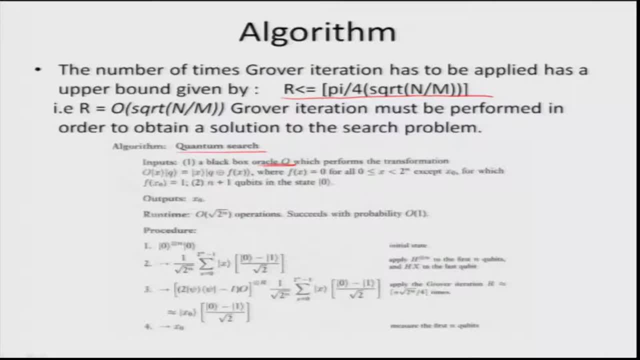 oracle O, which performs the transformation as given in this function, such that when the function has some values except the one that this, it is going to set up the value of f? x as 1.. Otherwise it will have the other answer: f? x equal to 0 and there are n plus 1 qubits. 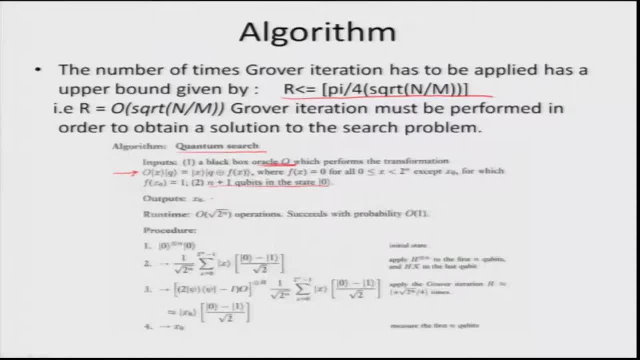 in the state, which is 0. The output is going to be the function n plus 1.. x- 0, which is your solution, and the run time will be of order. in this particular case, order 2 to the power n operations. It succeeds with probability of order 1, which means it is almost. 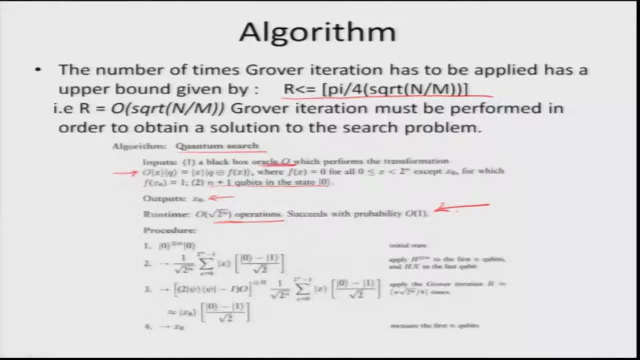 always it is going to be successful. It is just that there is a time bound beyond which it gets keeps on oscillating. So the procedure involves setting up the initial state and then applying a Hadley's equation, Android transform on the first n qubits and x to the last qubit, which is the result of. 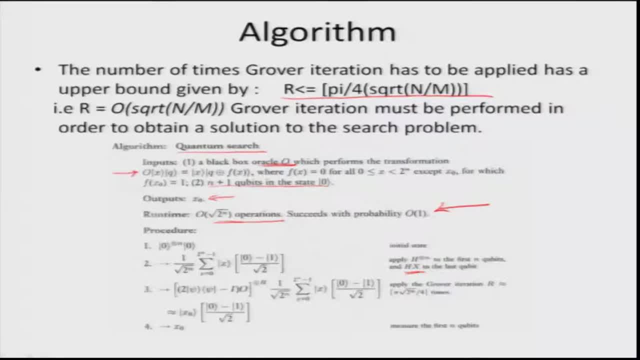 using the last qubit, x is the not gate, as we have said, and then we apply the Grovers iteration with r with this 2 to the power n over m. So we have basically chosen the special case where half of the our n by m is of the order 2 to the power m. So we get this and then, once we get the, 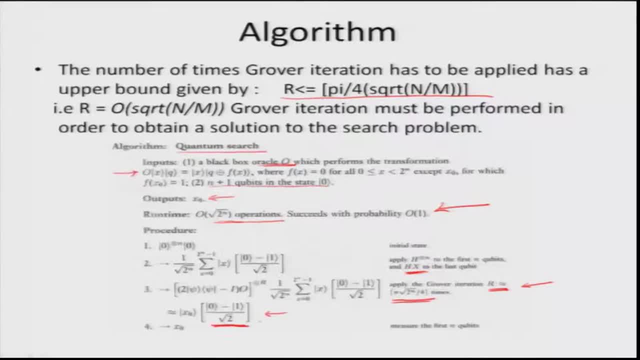 solution, which is of this order. this is our oracle qubit, So we preserve that, and our solution is X0, which is the first n qubits that we are looking for. So that is the basic algorithm behind the Grover's case, and here is how the circuit looks like. 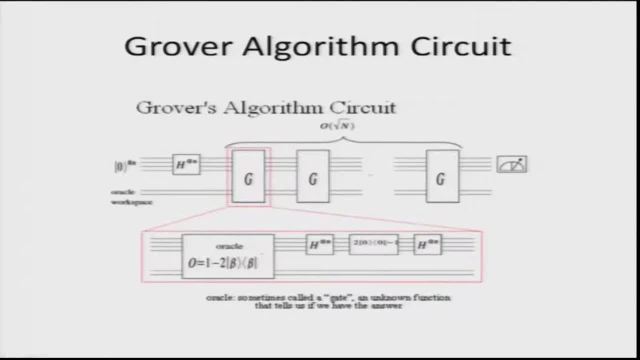 This particular case often is also known as a gate, as it is an unknown function which tells us if we have a function. So this is the oracle, which often, sometimes is also known as the Grover gate. in some cases is an unknown function which gives us, which tells us that. 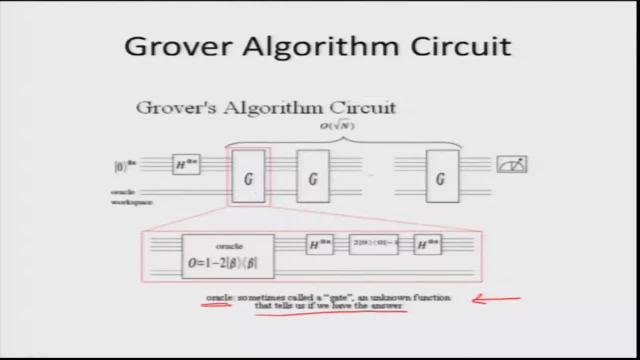 this if we have an answer. So this is how the Grover application of the Grover algorithm looks like the G gate or something, and this we apply it on the order of root n times and we should be able to get our proper solution and this is our measurement as we know this. 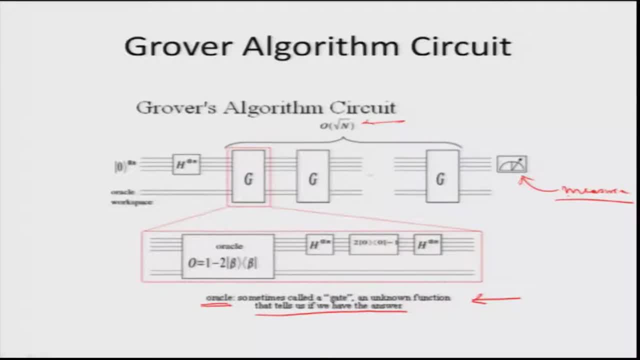 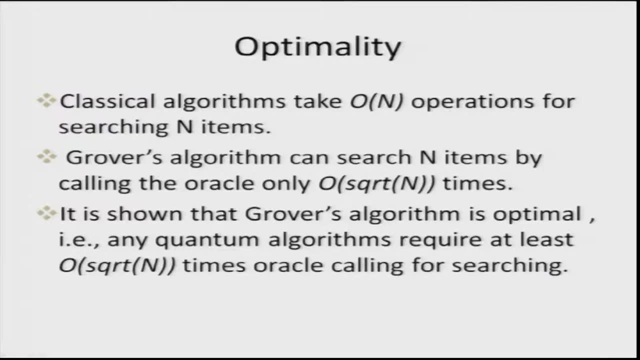 is what we have set up as our measurement state. The oracle work space always maintains the oracle qubit, which does not change as a result of this process. So one very important thing to note here as a result of this is the optimality of this. 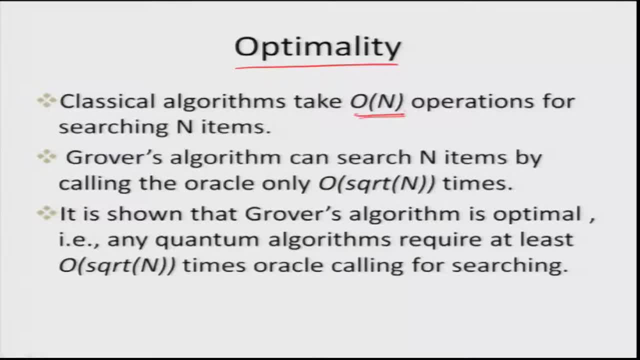 process. The classical algorithms take order n operations for searching n items. Grover's algorithm, however, can search n items by calling the oracle only square root of n times, And so it is at least quadratic speed up. It is also shown that Grover's algorithm is optimal, that is, any quantum algorithms. 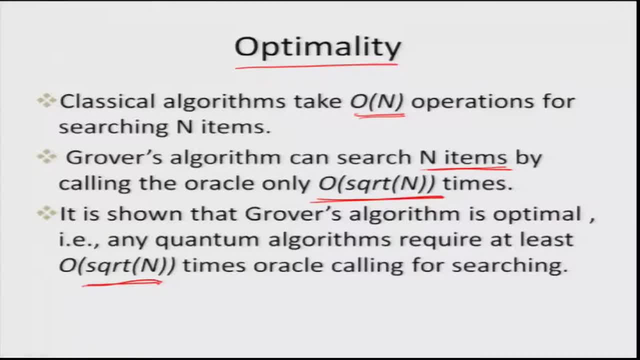 requiring at least square root of n times of the oracle calling for searching. and one of the important things, however important to mention here- that this entire picture is essentially true when it is an unstructured data set. This is because if you have already gotten a data set which is sort of structured in 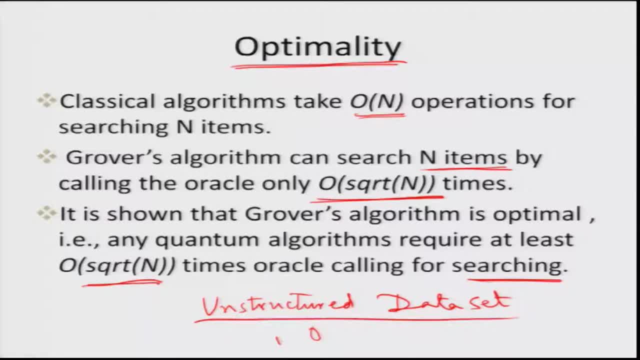 the sense that it is ordered. If it is ordered in some way, say from higher to lower numbers or something like that, Then the this idea of benefit from the Grover's search does not exist, also because in that case the operational procedures required to find the solution is of a different kind. 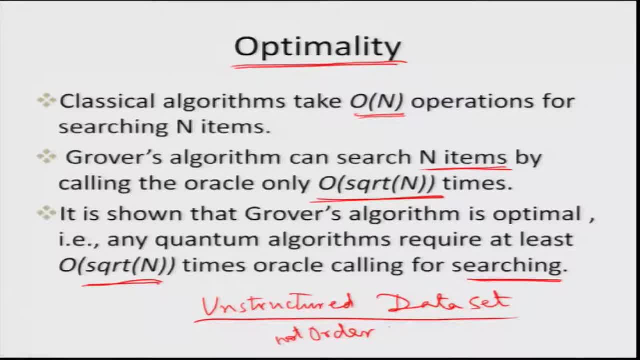 In most cases, for instance in case of classical case, you, if you have the prior knowledge that this data set is structured in some way, you will not have to look through the entire data set And therefore the optimality For the advantage that is required or necessary and which comes from Grover's algorithm, is: 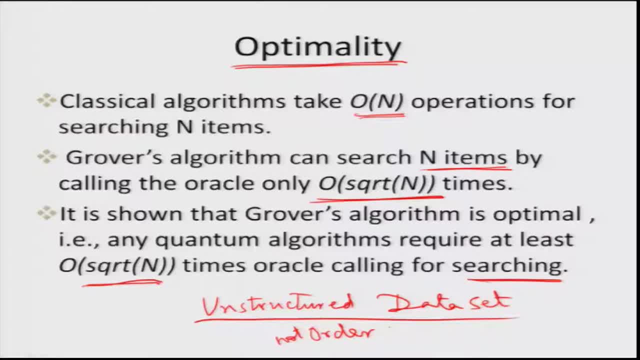 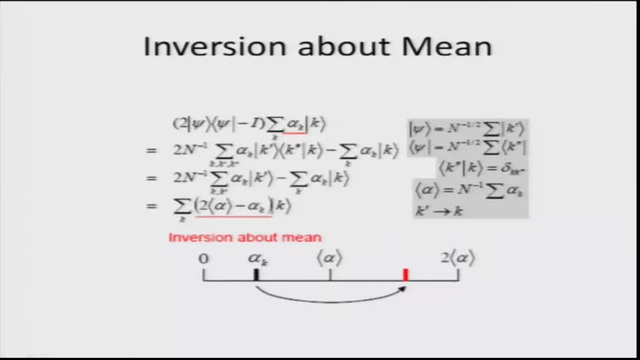 absent And therefore there is no benefit in that sense when we use the other kind of data set. So this particular algorithm is hugely effective in the case of unstructured data set. So that is the main issue and a small note about this other step that I have been talking. 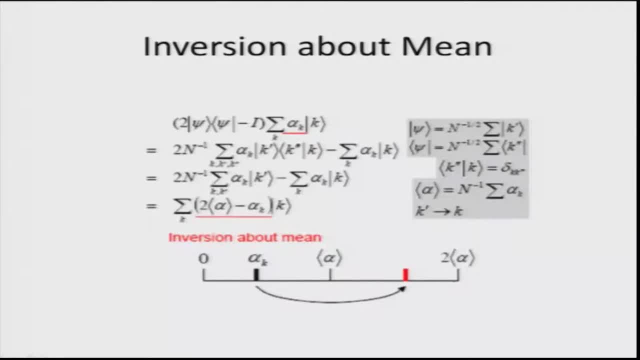 about Which is the. In this particular case, we are setting the value in such a way that everyone around the zero is going to change their sign, whereas the one at the zero remains the same, And that is where we have mentioned that the values go to minus. the case when it is about: 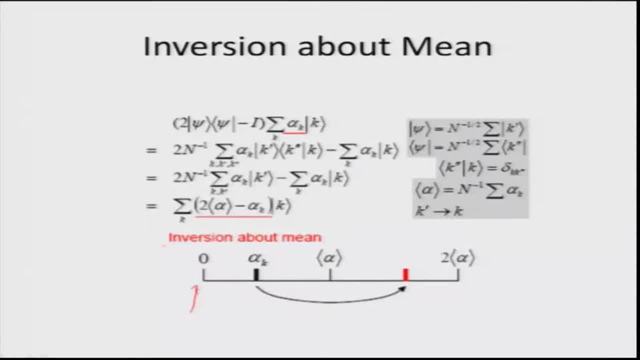 the zero values, otherwise it remains the same. So this is the inversion about mean. So for any data set, that is one of the steps that we have used. What we have done is that around the mean position which, for example, is this case, alpha- any number which is around the alpha, mod, alpha, or the mean value. 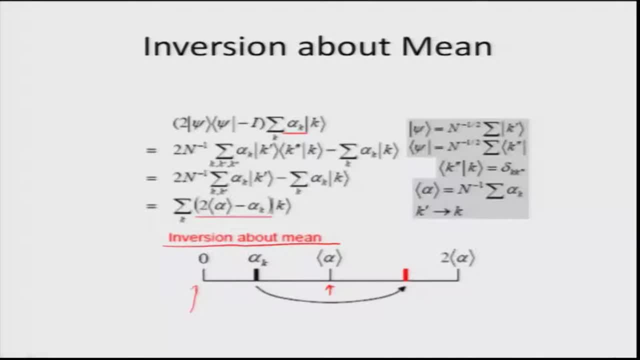 It will be changing its value, Whereas if it is on one side of it, will be remaining the same. So that is the idea about inversion of the mean, also applied in this case really effectively to able to mark out the right point. So what we have done today, 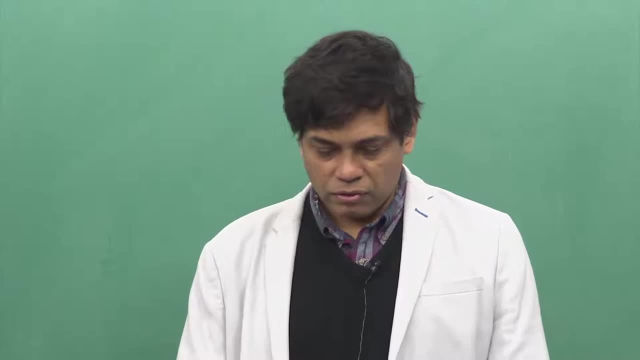 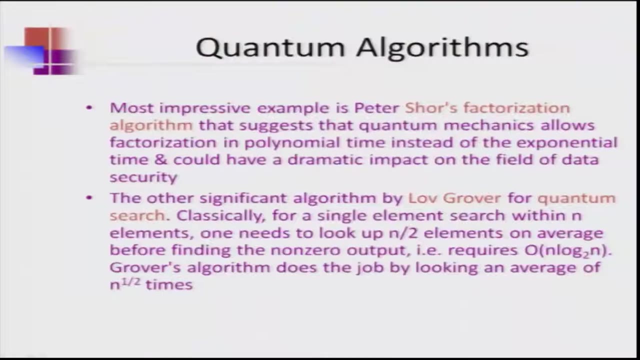 In today's class. I think I was good. Yeah is we have gone through one of the very basic algorithms but one of the very important algorithms which was discovered by Love Grover for quantum search, and it turns out to have at least a quadratic improvement over the earlier, over the classical search algorithms.